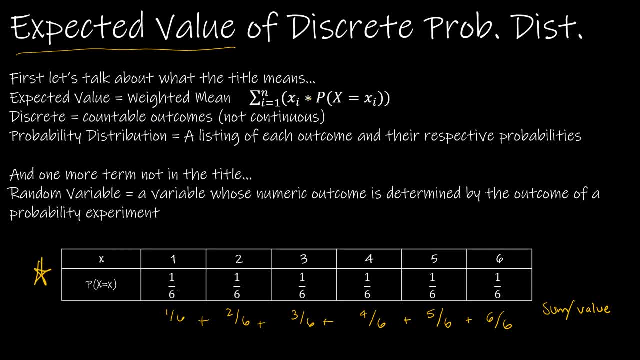 And a probability distribution is this: Here It's all of the outcomes and their respective probabilities. Now, one thing that I want you to really understand and I'm going to stress to you over and over, and you will probably get very sick of hearing me say: 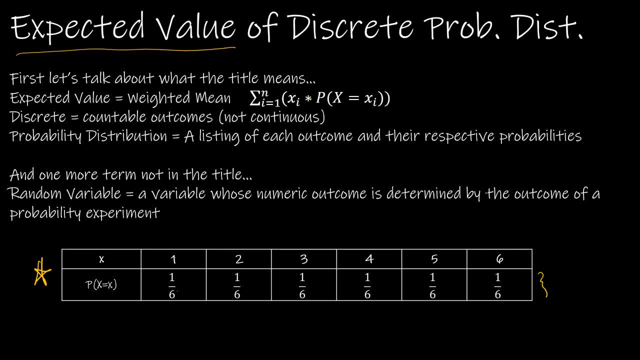 the sum of this has to equal 1.. Each of the probabilities. as we already know, each probability has to be between 0, and 1.. We've already talked about that property of probabilities, But this is very important. The sum of everything in the probability row- or column, depending on how you do it- has to equal 1.. 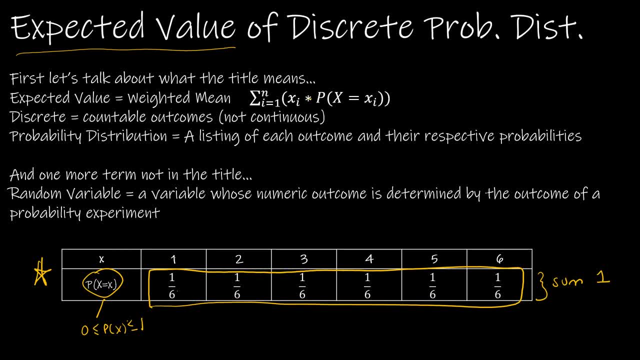 And if it doesn't, then it's not going to work to find the expected value. The last thing that I want to talk about, before we look at any examples, is another term called a random variable, And a random variable essentially is a variable whose numeric outcome is determined by the outcome of an experiment. 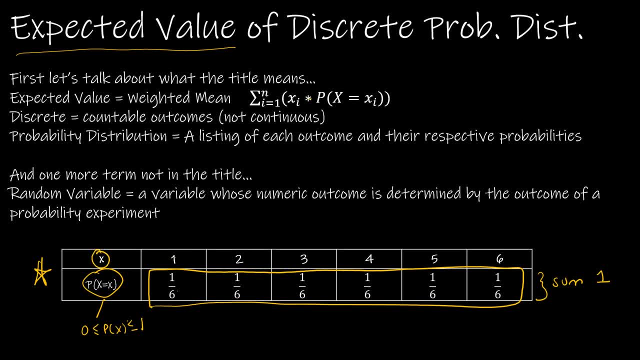 And what I mean by that is, we're using x to represent the outcomes of 1,, 2,, 3,, 4,, 5, and 6.. So x is our random variable that can take on one of these values. 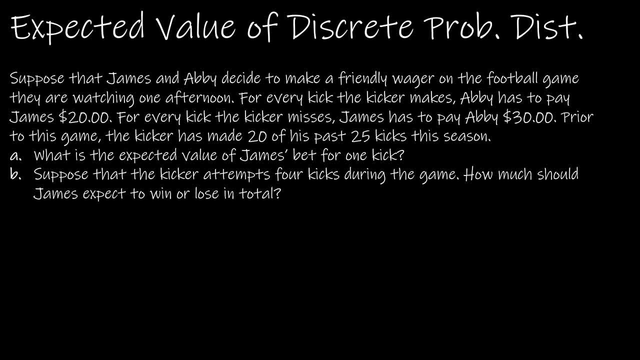 So let's look at an example together where we can find the expected value. So James and Abby are going to make a friendly wager On a football game they are watching one afternoon. For every kick the kicker makes, Abby has to pay James $20.. 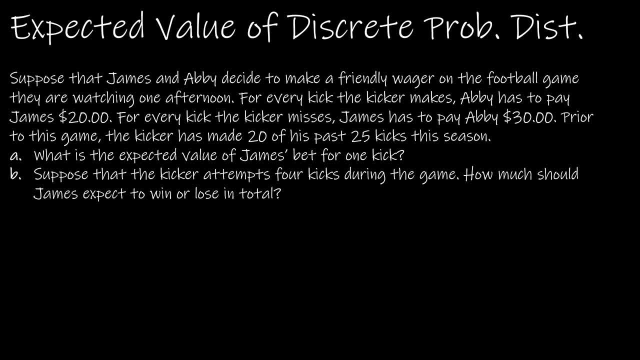 For every kick the kicker misses, James has to pay Abby $30.. Prior to this game, the kicker has made 20 of his past 25 kicks, So what's the expected value? So, really, what we want to do is we want to think about. 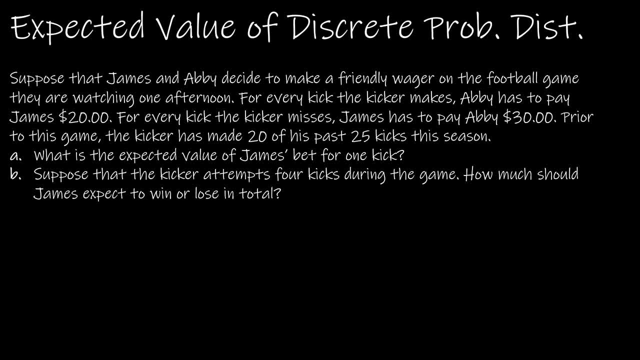 And again, this is for James. It says what is the expected value of James's bet. So if we were doing this for Abby, it would be the exact opposite. But let's go ahead and look at this, And I have done this ahead of time. 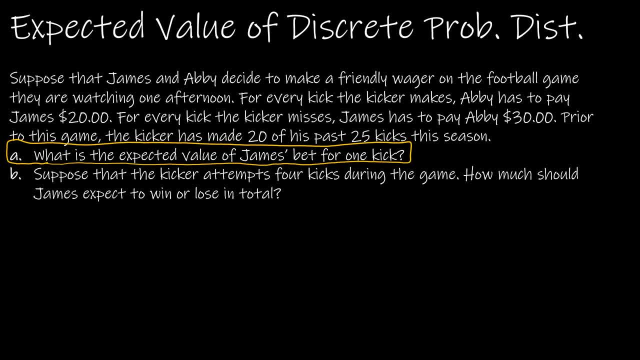 but we're going to work through it together. So what are the outcomes? The outcomes are make and miss, And again I'm thinking about in terms of James, if, and that's not even our x. so this is just the outcome. 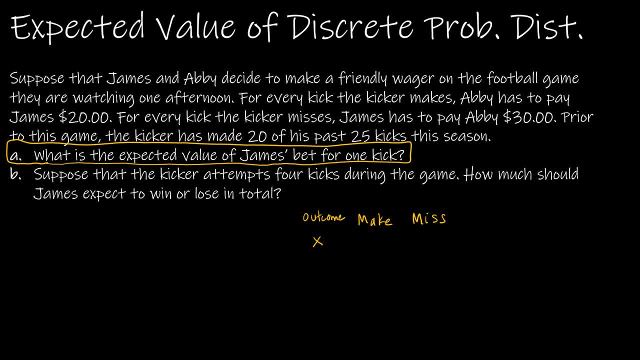 So if the kicker makes the kick, what happens to James? Well, forever. So every kick the kicker makes, Abby has to pay James $20, which means James just got $20.. So positive 20.. For every kick the kicker misses, James has to pay Abby $30. 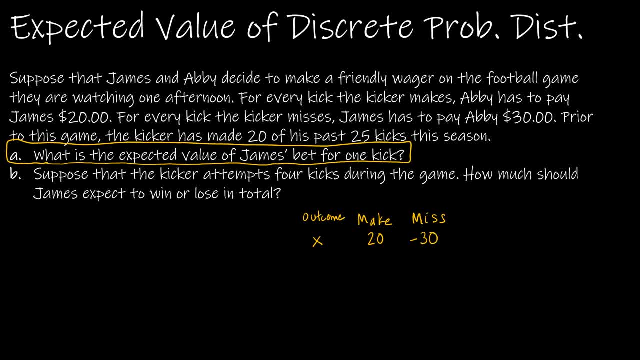 So on a miss, he pays $30.. Now, what is the probability? The probability that x is equal to x And again, x is either the 20 or the negative 30. So the probability of a make is. we're going to use the experimental probability. 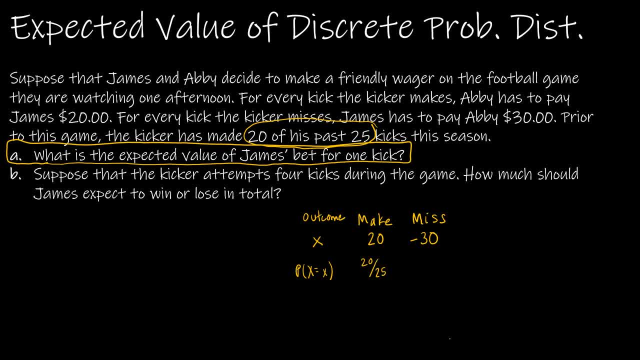 of 20 out of 25.. And then here's where that comes into play, where I said: this is always equal to one. So if 20 out of 25 is make, then five out of 25 is miss. So let me get rid of that. 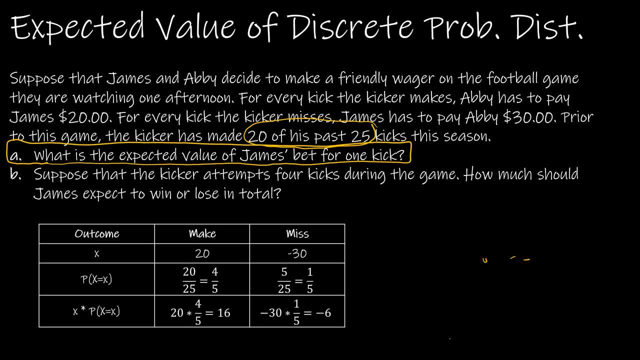 so you can see a much better indication. So again, what I have is the outcome is make and miss the 20 and negative 30. I have 20 over 25 and 5 over 25.. And then what I did was I took 20 times four fifths. 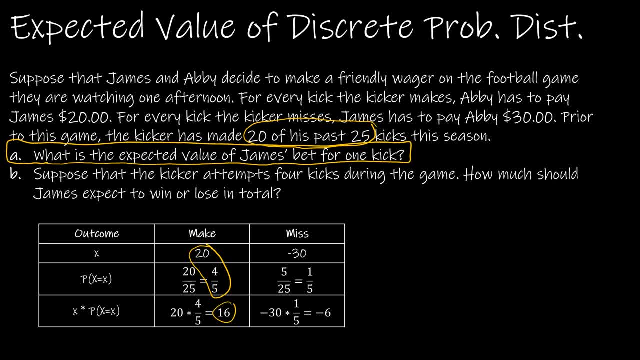 because I reduced 20 twenty-fifths to four fifths and that gave me 16.. And then I took negative 30 times one fifth, which is negative six. So what's the expected value? The expected value, which is just E of x. 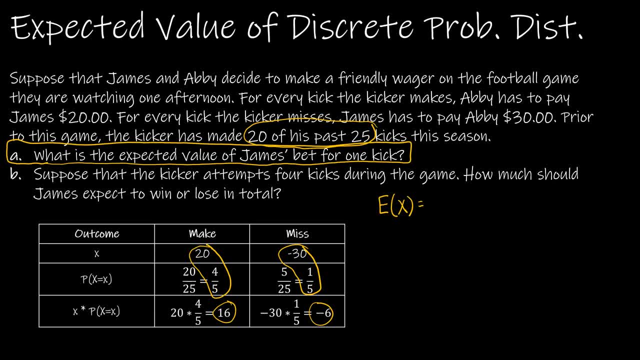 is how we denote. that is x, the sum of all of these. so the sum is 16 plus negative 6, which is 10. what does that mean? so, before we look at B, what does that mean? that means every time the kicker kicks the ball, we expect James to make $10. now again. if we did this, 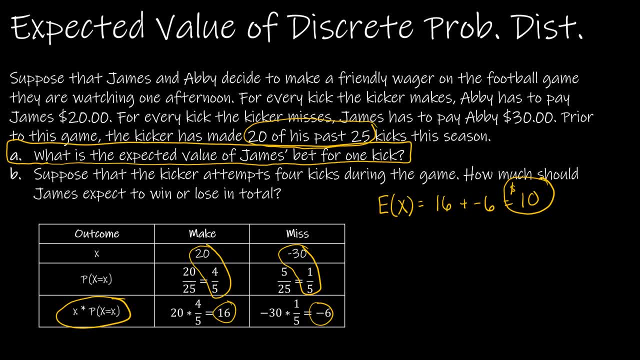 instead for Abby. we would say that every time the kicker kicks the ball, we expect Abby to lose $10, and we're not going to go through that one. but it would look very similar to this: it would just be a negative 20 and a positive 30 and that. 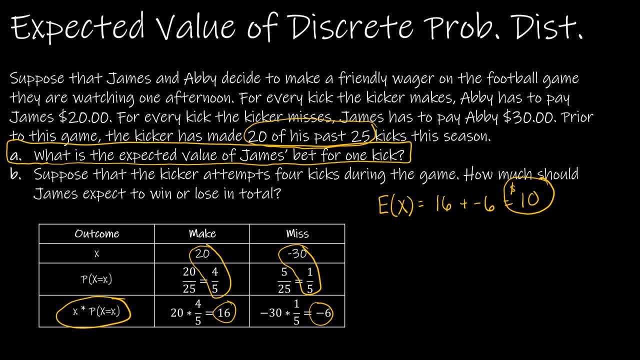 would give me a sum of negative 10. so the next question says: suppose that the kicker- I'm going to change colors. suppose that the kicker attempts four kicks during the game, how much should James expect to win or lose? so if we have $10 each game, then we're just going to take four times. 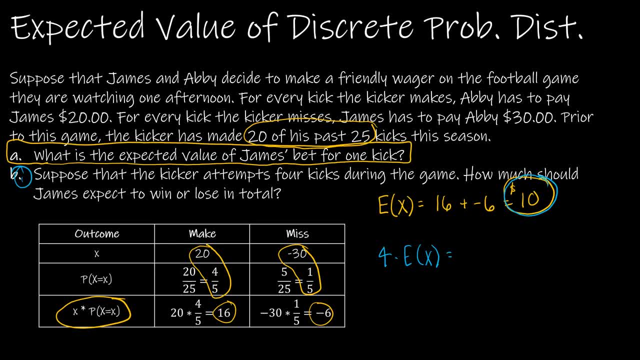 the expected value because we're playing four- or, I'm sorry, he has four kicks. not four games, but four kicks. so we're going to take four times ten, which is 40. so at the end of the game James should expect to win $40, because he wins on average. 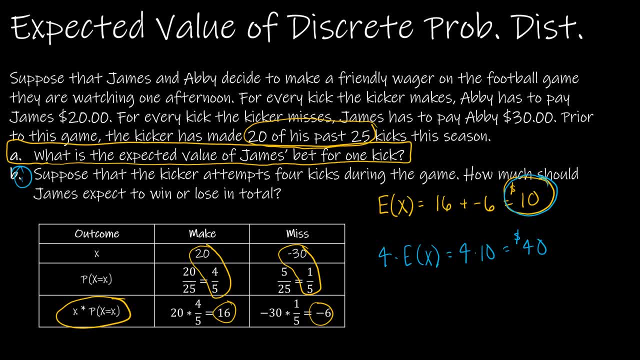 $10 every time the kicker kicks. now a lot of people struggle with expected value because they say, well, there's really no way to get exactly ten dollars, and in this case there is. he could make twice and miss once, but you get the idea that we're. 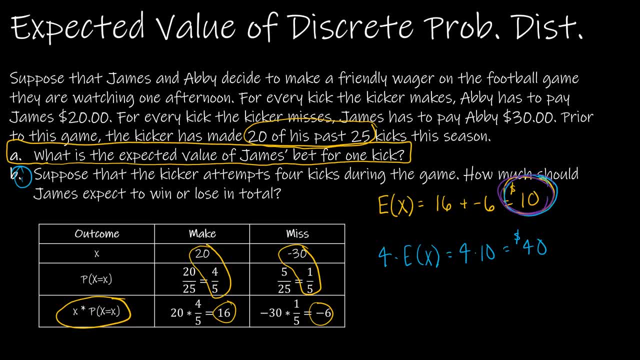 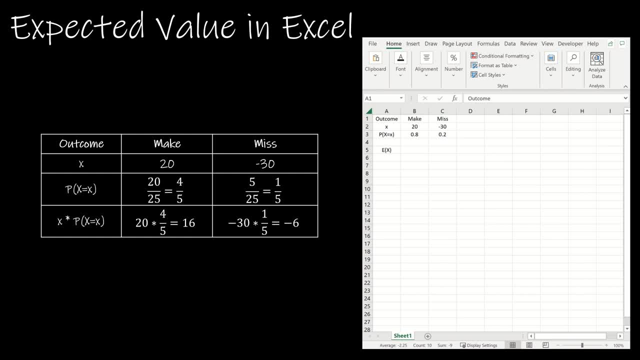 looking at averages. we're just looking at averages, a weighted mean. I want to take a look now at how we can allow Excel to do the calculations for us. so, as you can see, all I've done is I've copied over the information. outcome: make miss for X. I have positive 20. 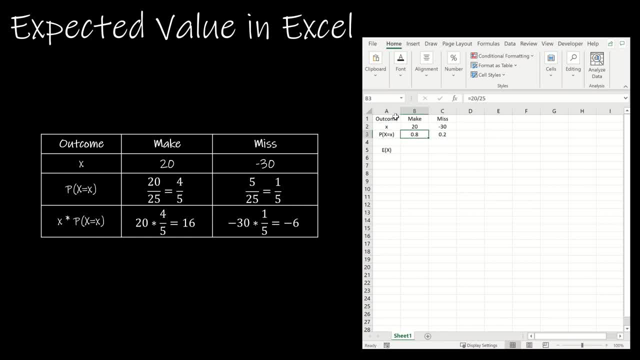 negative 30 for the probability that X equals X. I simply used equals 20 divided by 25, so there's no need to reduce that fraction. just let Excel calculate the decimal for you and then equals 5 divided by 25, which is 0.2. now I want to. 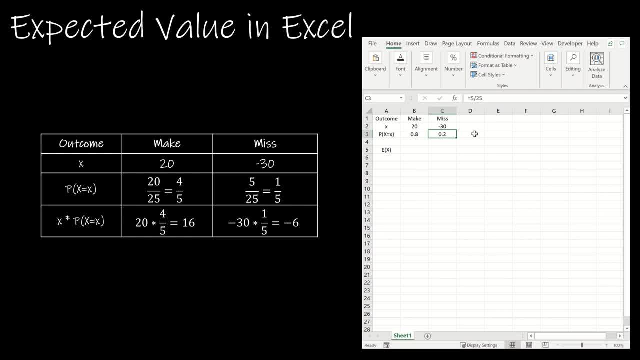 encourage you before I show you how to do this in Excel. I want to encourage you to not round. so I have a lot of people who try to round these two values and when you round in the middle of a calculation and make sure overall result less precise, so don't do it. so in order for 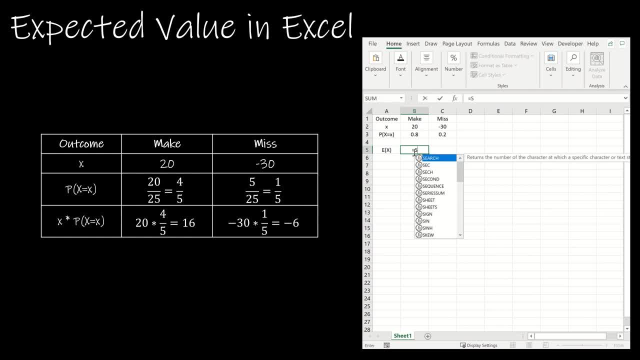 me to find the expected value. I'm just going to use that some product function that we've already learned when we talked about a weighted mean. so my first array, and here's the important part, I need to make one of the arrays the X's and one of the arrays the values of zero. so here's how you can do. 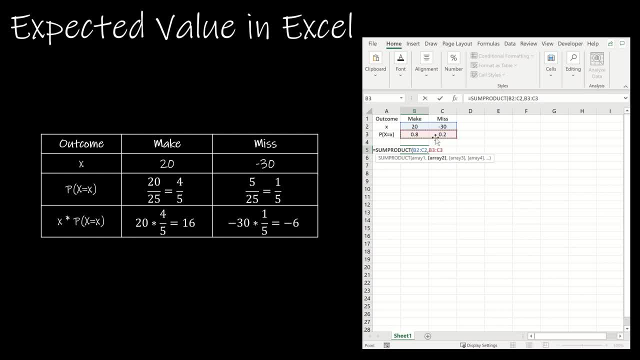 and then comma, and then one of the arrays, the probabilities. So I'm not going to get the right answer if I take 20 and 0.8 in one array and negative 30 and 0.2 in the other array I need. 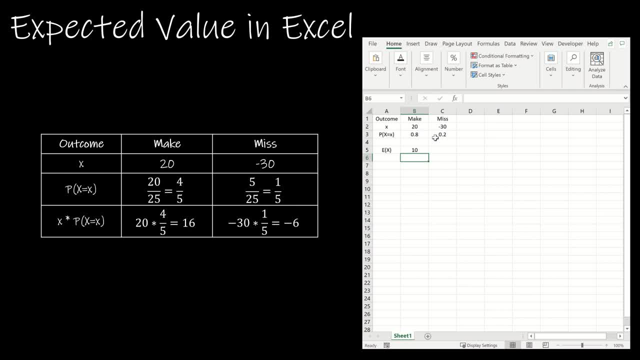 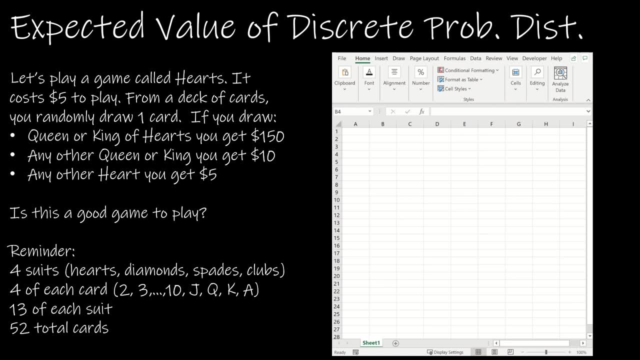 to keep like things together And notice I got my expected value of 10.. Let's take a look at another question together. As you can see, I don't have anything filled in on my Excel spreadsheet because this is the kind of question that you're going to get that you'll need to work through and 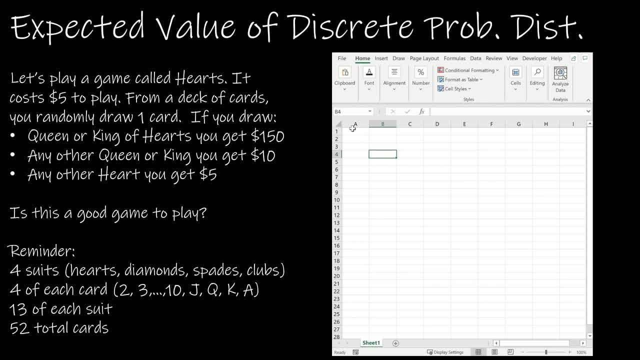 create the spreadsheet on your own. So let's talk about how to do it. Just as I did before, I'm going to come up with the outcomes, the result of that outcome, I guess you would say, and then the probability that x is equal to x. So that's what I'm going to come up with for each one. 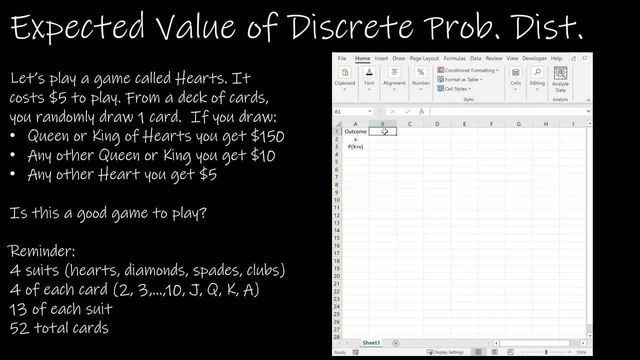 And in this game we have a game called hearts. it costs $5 to play. From a deck of cards you randomly draw one card. If you draw a queen or king of hearts, you get $150. So my first outcome is queen or king of hearts. My next outcome is other queen or king. My next outcome is: 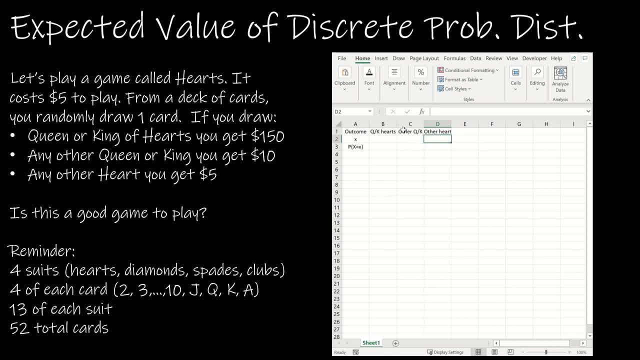 other heart And a lot of students stop right there and say: well, that's all the ones that you live in right listed for me, So that must be it. So hopefully you know that's not the case, But just in case. 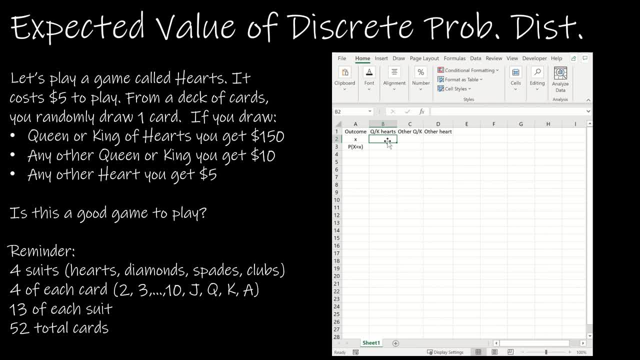 that was you. let's talk about how we know that's not the case For X. I'm going to write down what happens to me, what happens to my pocketbook when I get a queen or king of hearts. It says I win $150.. But if you'll notice, it does cost me $5 to play. So my overall outcome. 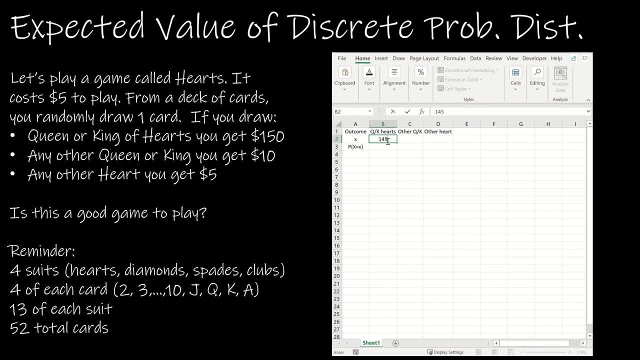 is that I win $145.. For any other queen or king I get $10. But again it cost me $5 to play, So I get $5.. For another heart, I basically break even. I get my $5 back, So I didn't pay anything. 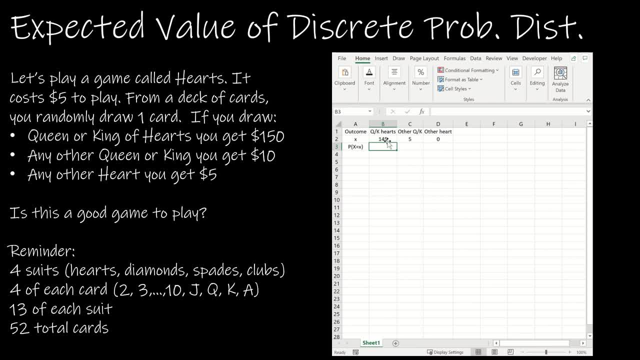 Now for the probabilities. again. I've put a reminder for those of you who are not card players. For the queen or king of hearts I'm going to use the equal sign. there are: there's one queen and one king, so that's two cards out of 52 total cards for other queen king. that's the queen. 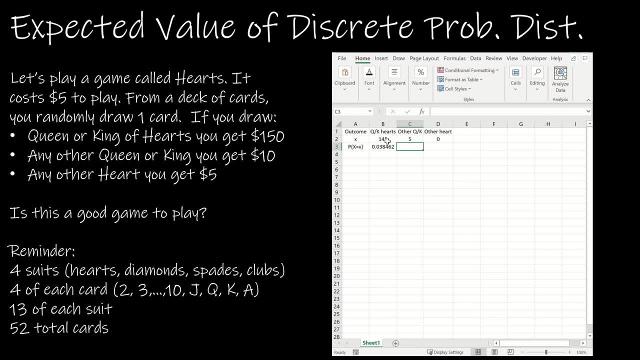 or king of diamonds, queen or king of spades, queen or king of clubs, so there are six of them out of 52. and for another heart, remember there are 13 of each suit, so there's 13 hearts. but i have already used the queen or king of hearts to win my 150, hopefully, so there are 11 cards left, so equals. 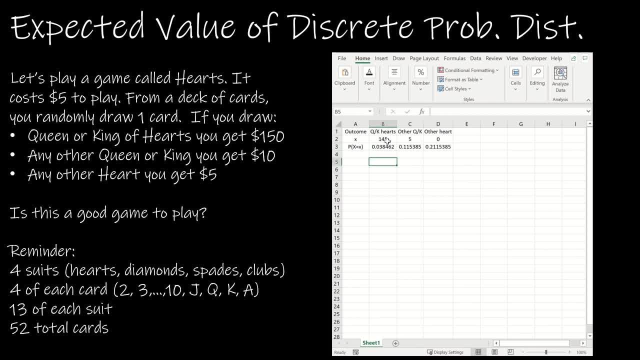 11 out of 52. now, here's where you have to be careful, because a lot of students stop right there and then they say, okay, the expected value is equals some product, and then they take this array and i'm going to go ahead and go one more and this array and, if you'll notice, i get six. 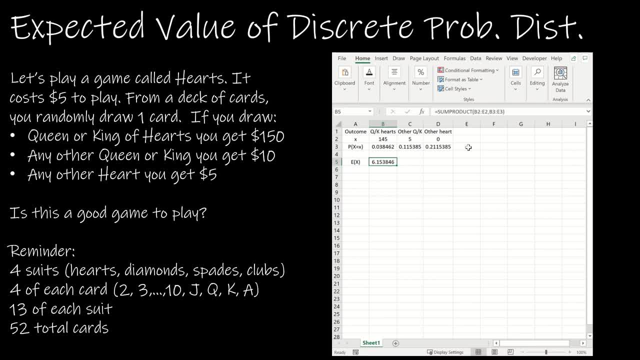 dollars and 15 cents, which basically means every time i play, i win six dollars and 15 cents. so sure, yes, i obviously absolutely want to play now. the problem with this is that i'm going to find the sum of the probabilities and the sum of the probabilities- remember, it needs to equal one and right now, the 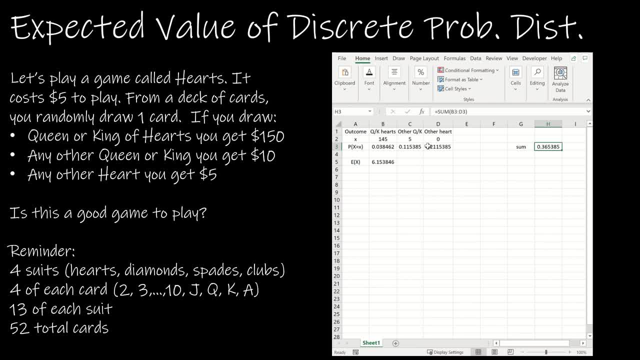 sum of the probabilities equals negative, i'm sorry, equals 0.365385, not one. so i need essentially any other card, so a card that we haven't mentioned yet. if i get one of those cards, i lose five dollars negative five. so what's the probability? well, i can either count up which cards i haven't used, which is. 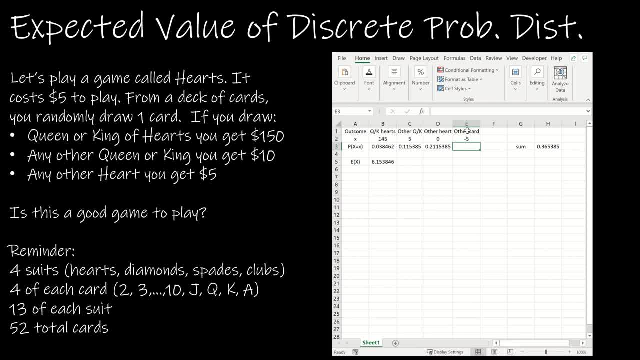 all of the diamonds, all of the spades, all of the clubs, except for the queen or king, which would be 11 for each, so 33 cards. and then i could say, okay, does that then equal what i need it to equal? and it does. the other way i could have done it if i don't want to think that hard abcd. 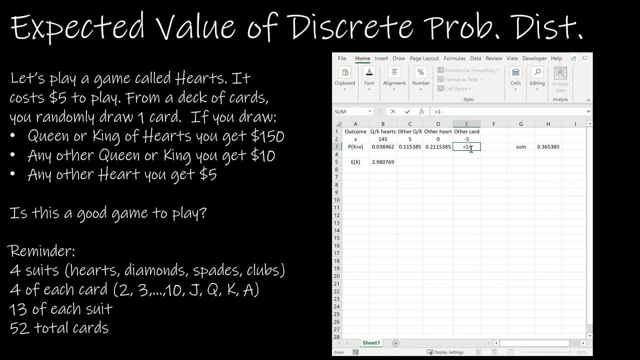 is. i could have just said equals 1 minus whatever the sum is, and notice, i got the exact same value. so what happened is now my sum of all four columns is equal to one, but the sum of the three plus the sum of the other, so the other card was just one. 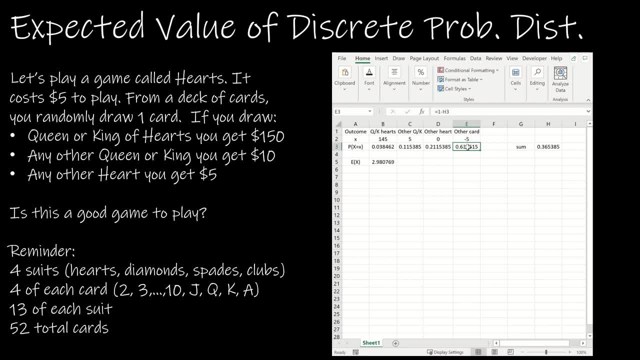 minus because, again, the sum of the probabilities must equal one. now, is this still a good game to play? well, how do we know to determine if this is a good game to play? i need to look at my outcome. did i win money? well, i did. every time i play this game, i'm supposed to win 2.98. and again, if you want, 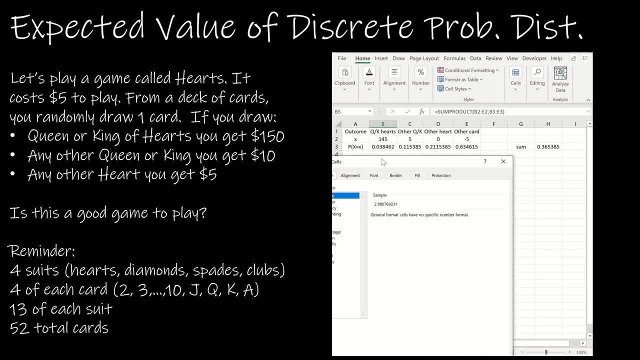 to. you can go to format cells and you can say that this is a currency and go to two decimal places. so two dollars and ninety eight cents is what i expect to win. now a lot of people stop here and say, well, no, that's not true, because i had to pay five dollars to play and so i'm actually losing. 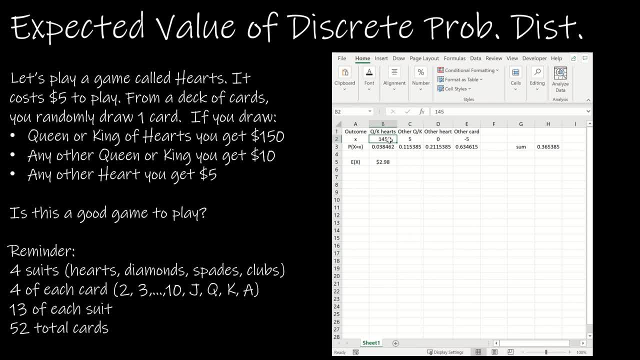 money, but, if you'll recall, we already took the five dollars into play here, here, here and here. so this is a great game to play. every time i play the game, i should win three dollars. so if i play this game a hundred times, i'm up 300 bucks on average. 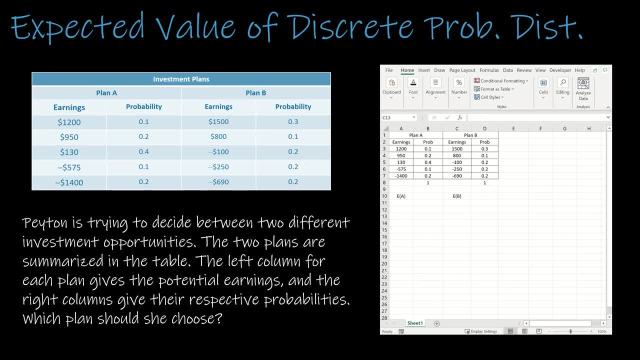 here's a question i would like for you to try on your own. there are two different um investment portfolios that peyton could- uh could- invest in, and she's trying to find the best option for herself. she's going to look at the earnings, or the expected earnings, for each of those plans and shoes. 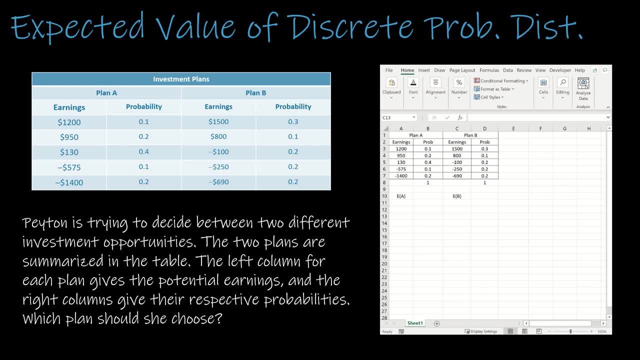 based on the expected earnings, and she's going to look at the earnings or the expected earnings for each of those plans and choose based on the expected earnings again. what we're looking for is a weighted mean. now i've already decided or shown you that the sum of the probabilities for each is equal to one. therefore, we can use that. 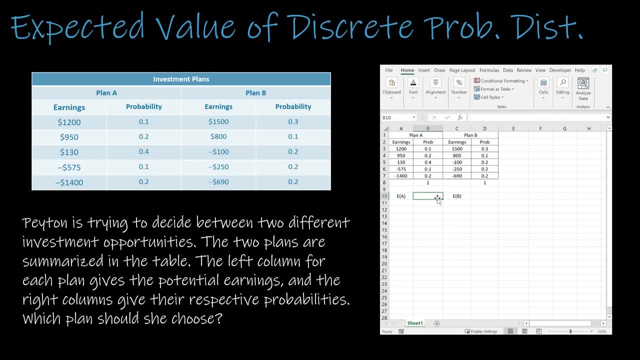 sum product function. so i would like for you to find each of the expected values. when you're ready and made your decision, press play to see how you did so. again, i'm going to look at the sum product function and choose what you've already done in the step by step process. 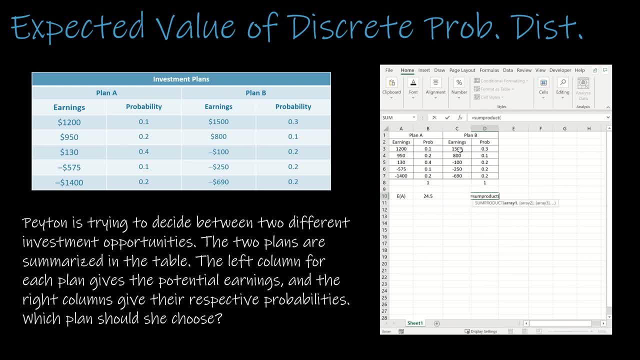 we're just going to run this through a series of options here. so here we go: choose one array to be earnings, one array to be probability, make sure that you have the same amount of values in each, and then some product here for earnings and for probabilities.